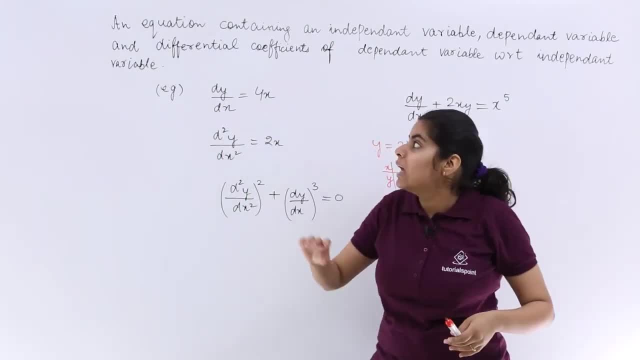 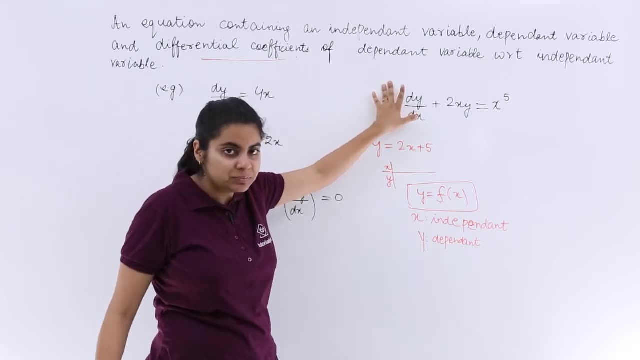 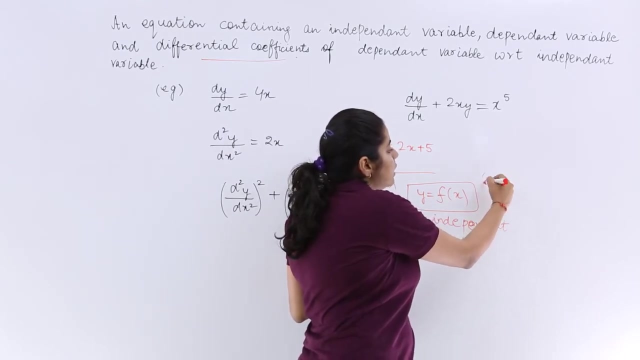 it contains independent variable, dependent variable and differential coefficients- This word is important- Differential coefficients of dependent with respect to independent. So if I say that dependent is y, independent is x, So differential coefficient is x, is d, of y upon dx, because differential coefficient of dependent over differential coefficient of 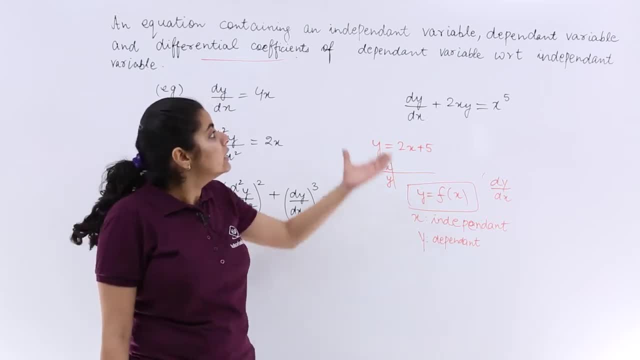 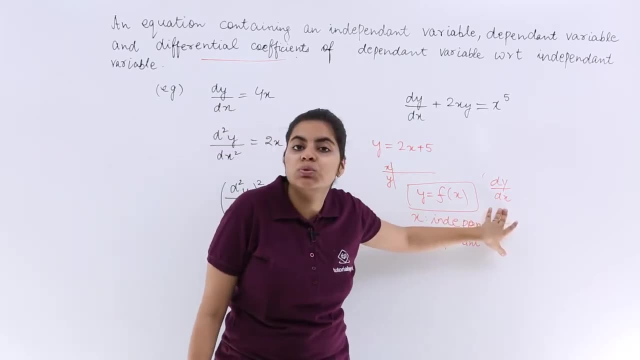 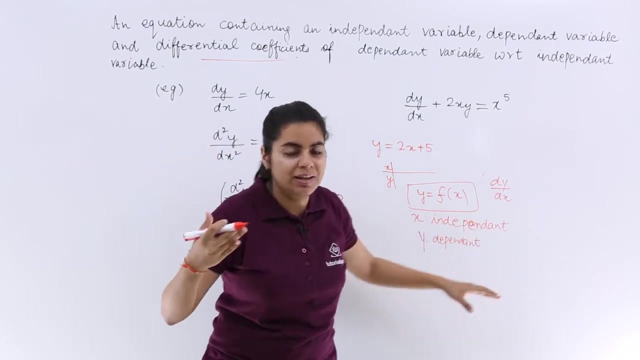 independent. The other thing. the other thing is that these have variable orders. that means it is not always dy by dx would be there. it can be d2y by dx square, d3y by dx- cube, and also there can be whole square, whole cube to that too. Let's take these examples. this is dy by dx is equal to. 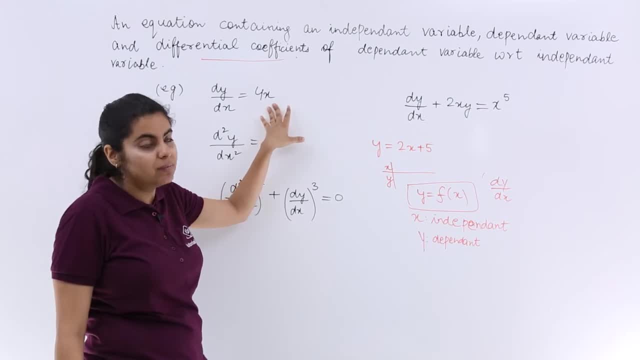 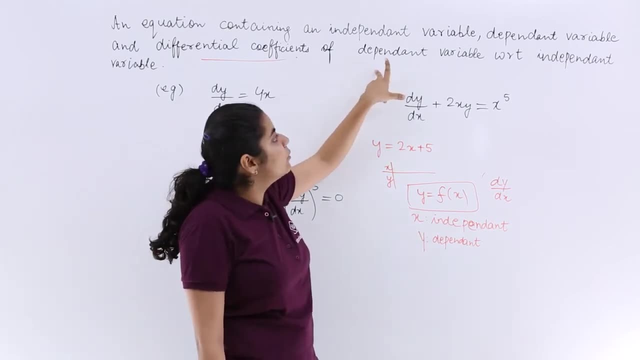 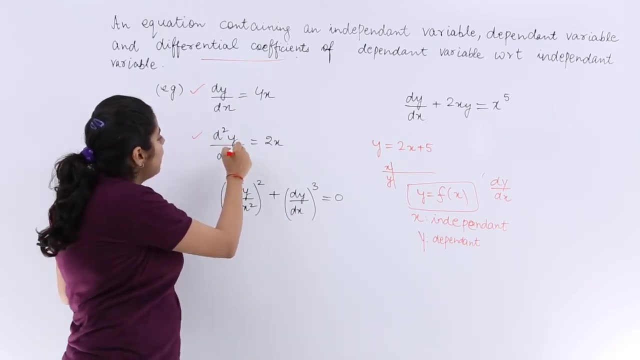 4x. so it contains x as the independent variable and dy by dx is already there. that dy by dx is differential coefficient of independent and dependent. you see that dependent with respect to independent. so this is a differential equation. Now here, d2y upon dx square is equal to 2x. 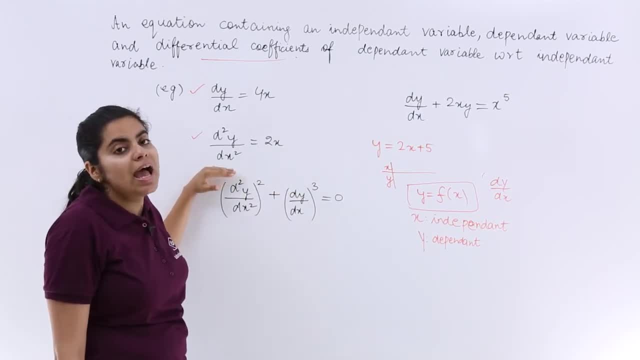 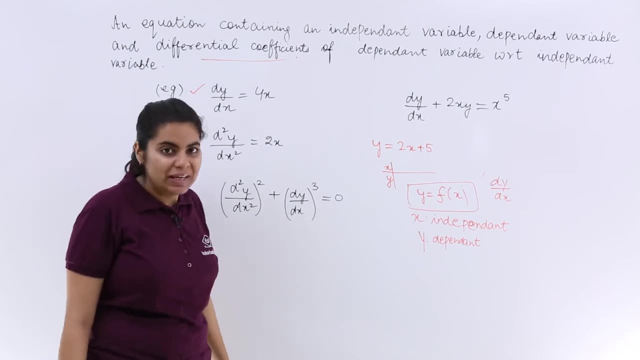 again, you see that here there is a differential coefficient, and you see, I told you, it is not always that dy by dx can be there. other variations are possible too. Next, you see this example: d2y upon dx square, whole square plus dy by dx- whole cube is equal to 0.. 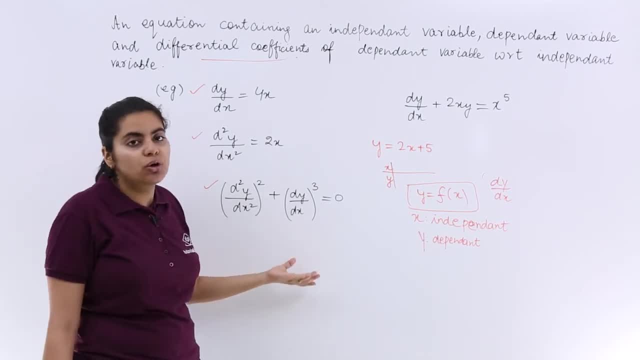 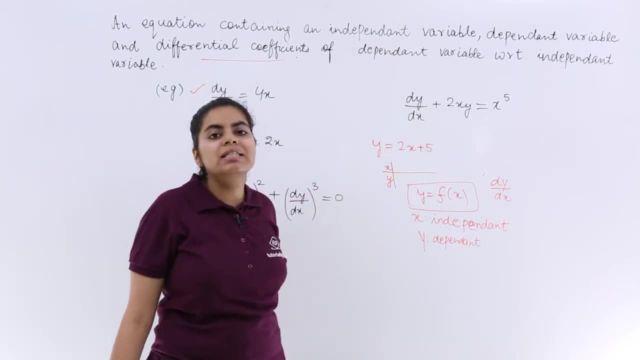 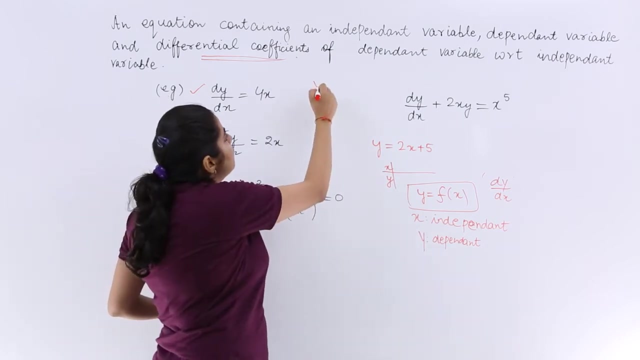 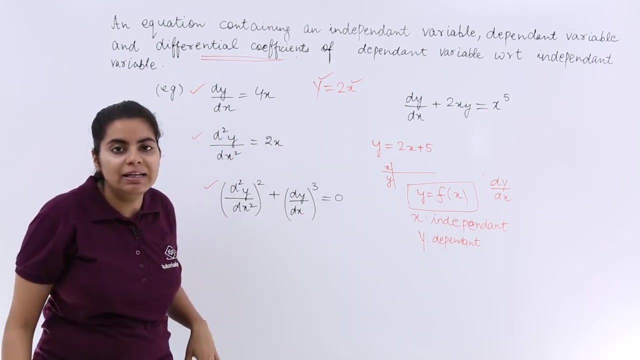 It is an equation has equal to, there are differential coefficient. so what is important? in a differential equation you may miss the independent variable and something parts like dependent, but differential coefficient will always be there, right? if I say y is equal to 2x, there is independent variable, there is dependent variable, but there is no dy by dx, until and unless you. 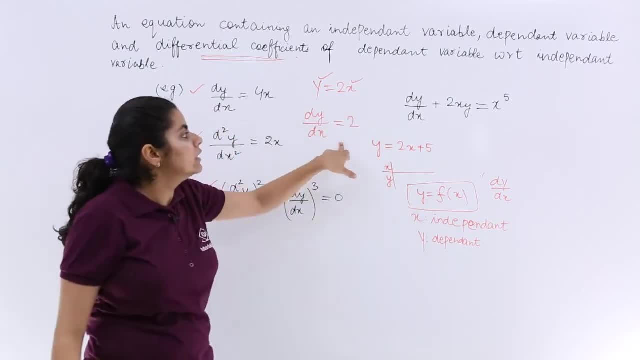 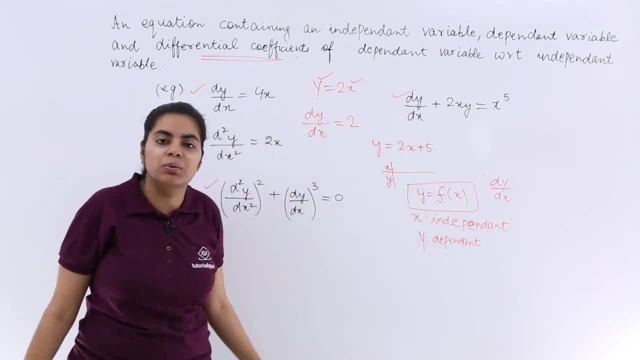 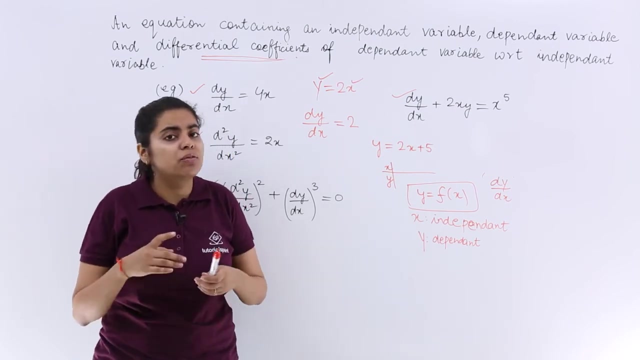 differentiate it and then you get like this: this is your differential equation, right? so next example is again: dy by dx plus 2xy is equal to x, raise to the power 5. so now you understand what is a differential equation, but we also need to know in what cases, or what would be the scenarios wherein-